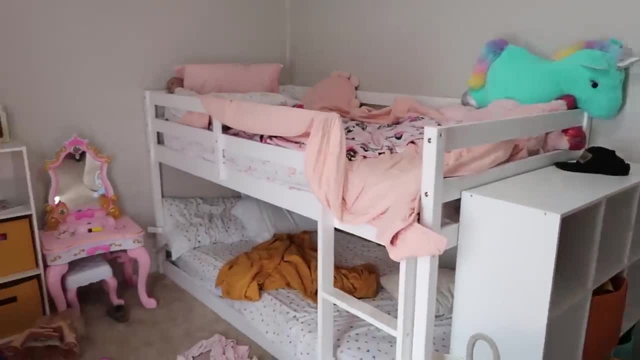 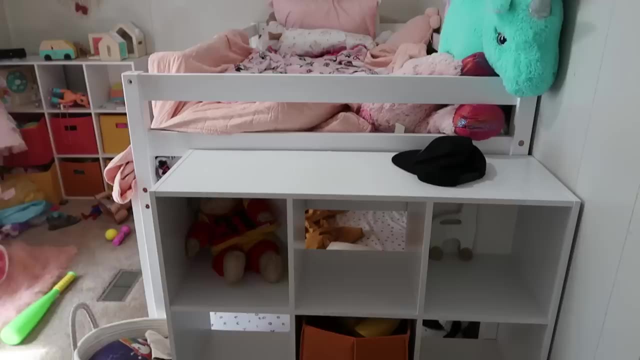 things so that I could keep them separated and they kind of had their own spaces. This worked out really well for a while, but it eventually just got to where all their toys were just getting mixed up anyways- and they're at the age where they play with each other's things anyways. So 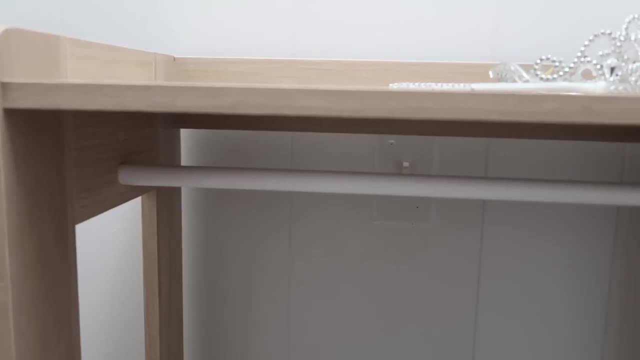 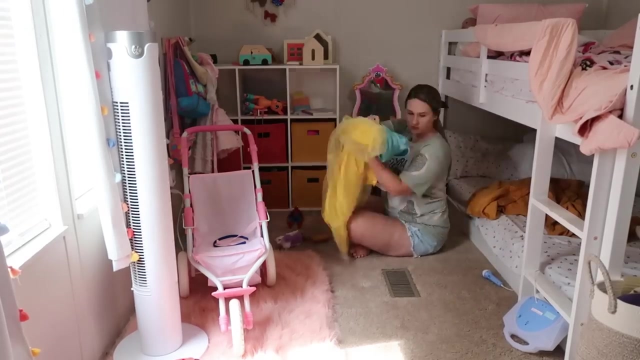 I'm going to be doing a room refresh. We're going to be adding in a dress-up closet. This is from Amazon- I will have a link down below if y'all are interested- and the little pom-pom mirror is from Target. Cleaning and organizing in a kid's room will never not be overwhelming, So I have learned. 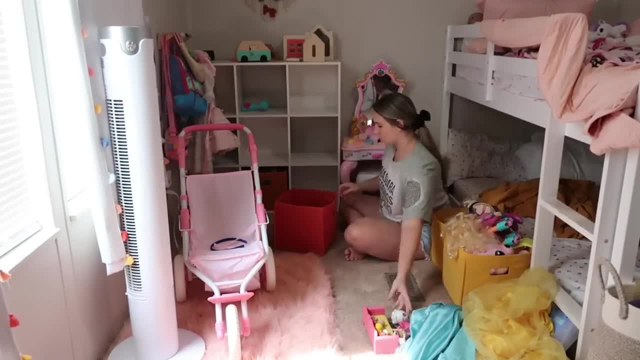 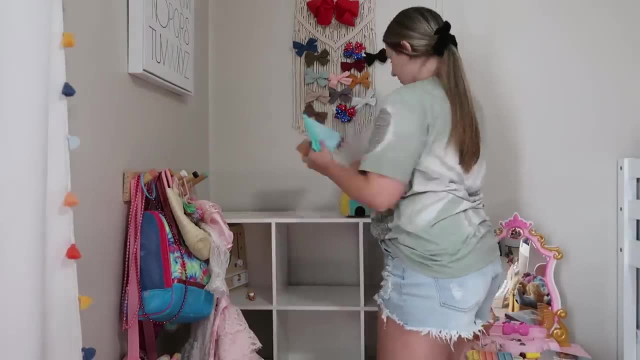 to start in one space at a time, so I'm going through each box one at a time just to make sure there's nothing in there that shouldn't be any paper. Sometimes I find the randomest things in my kid's room, so I'm going to go ahead and get anything out of here that's not supposed to be in. 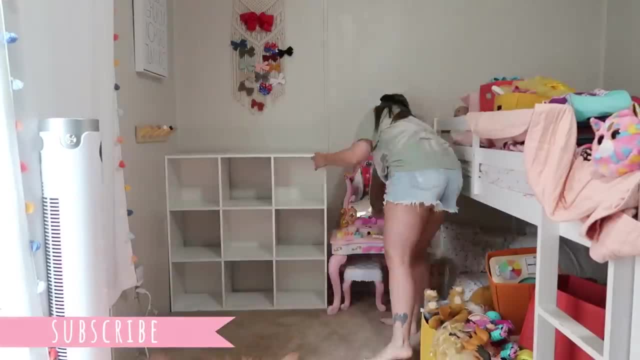 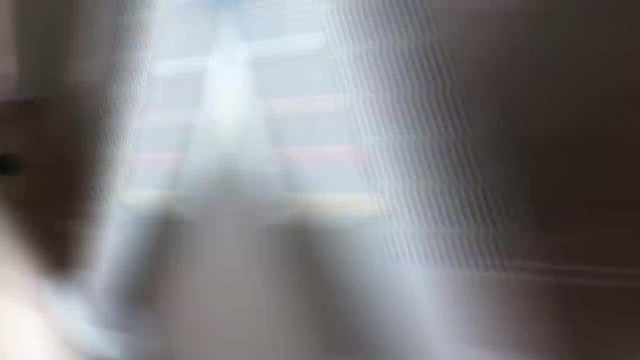 here. I'm going to be taking out this cube organizer and we're only going to be having one cube organizer for all the toys. I'm just going to mix their toys together, since they play with each other's toys anyways, and the dress-up closet is actually going to be so helpful because 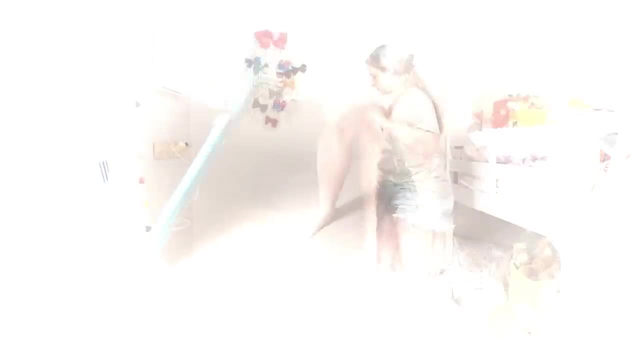 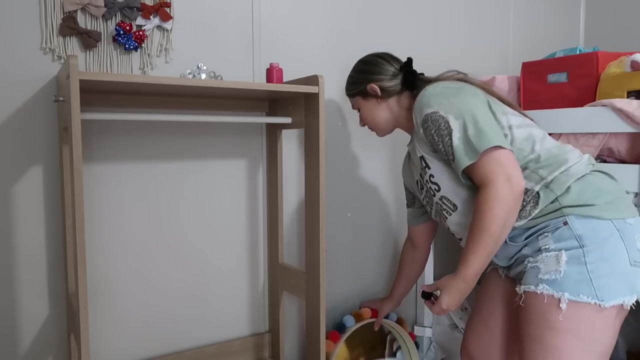 most of Arabella's toys is either Barbie or dress-up clothes. That's just what she prefers to play with. So, instead of having all the dress-up clothes shoved in cube organizers, we're going to be hanging them up and displaying them, and this 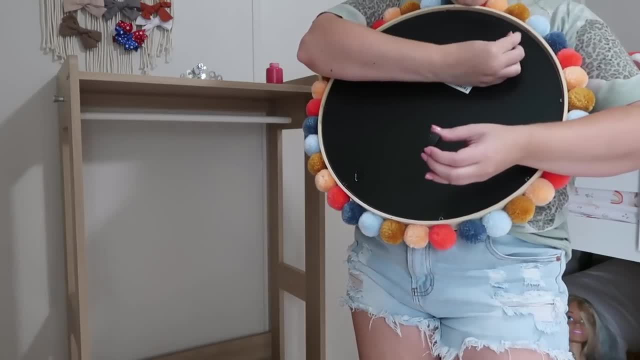 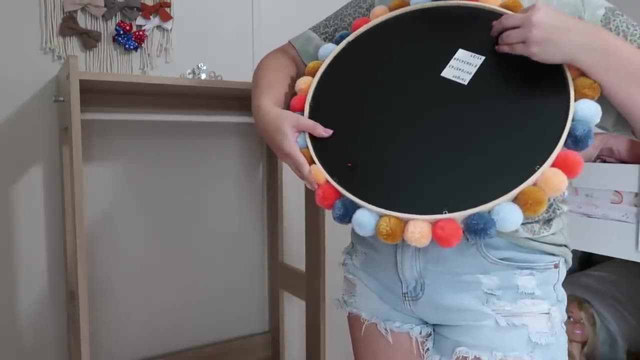 is also going to be for Nolan, my son, because he likes to play dress-up as well and he's got hats and sunglasses, So this is going to be useful for their Halloween costumes so that they can play dress-up. So what I'm doing here is taking a little bit of washable kids paint, dabbing it onto the 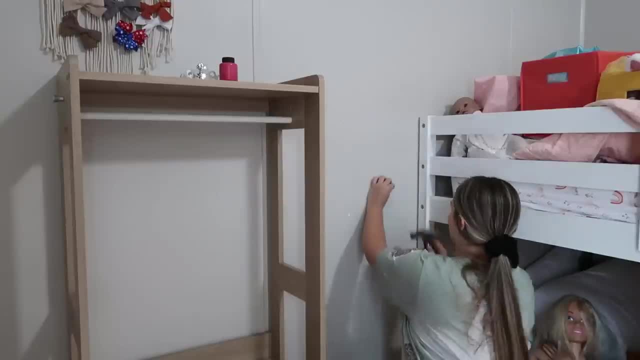 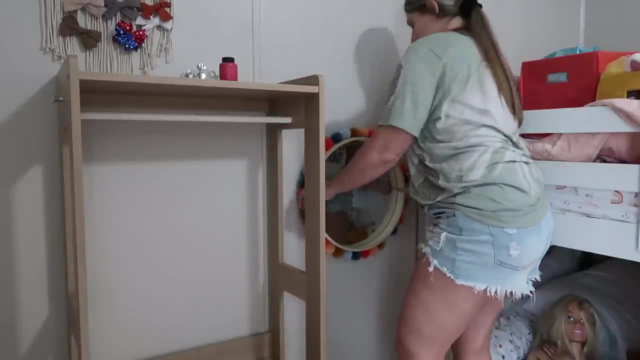 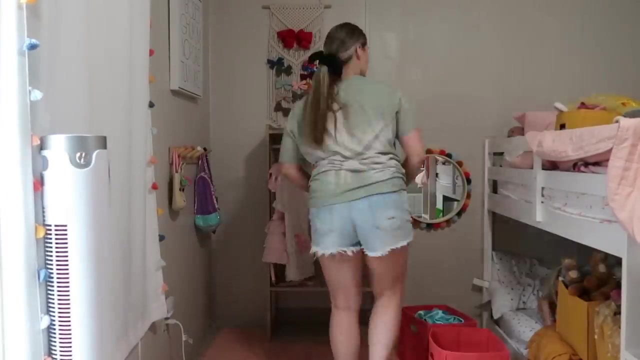 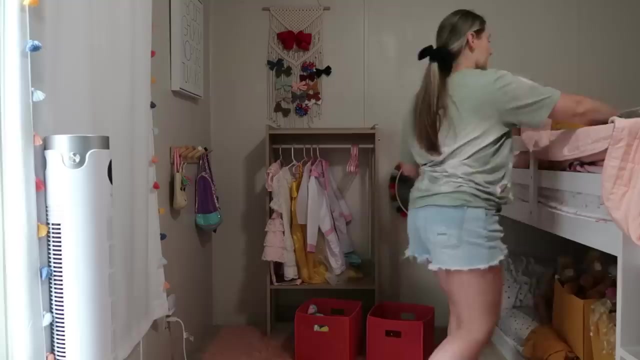 little hooks so that I can push it against the wall to see where I need to put the nails, and it works like a charm. If you have little girls, I really hope that I'm able to give you some inspiration for their dress-up clothes. This is such an adorable idea for their bedroom, or just put it in their closet. 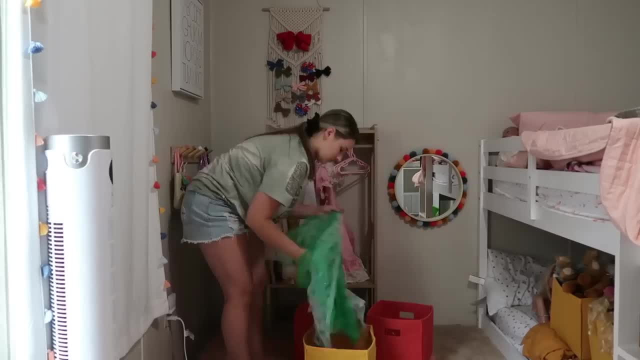 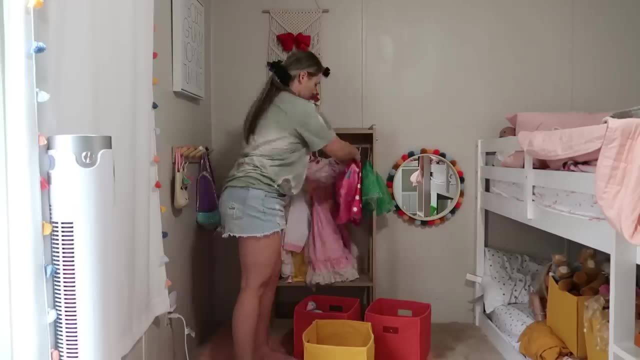 or use it in a playroom. It is such a wonderful idea to hang up their clothes instead of shoving them in toy boxes. and, yes, this is aimed towards little girls. but come Halloween, Nolan's going to have a new Halloween costume and I'm going to work on getting him some like firefighter and police. 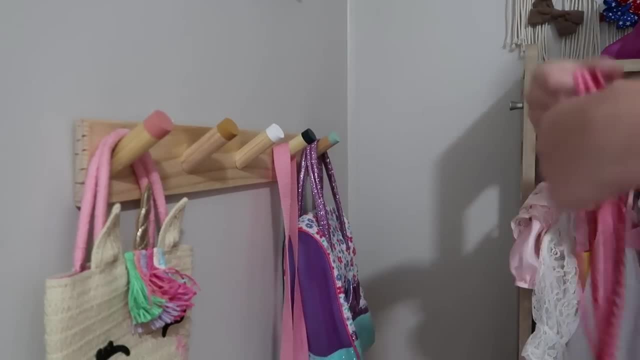 officer costumes and we're going to just make it so fun over here in this corner for both of them. but right now it does look pretty girly, but I do plan on making it a little bit more of a space for a little boy as well. 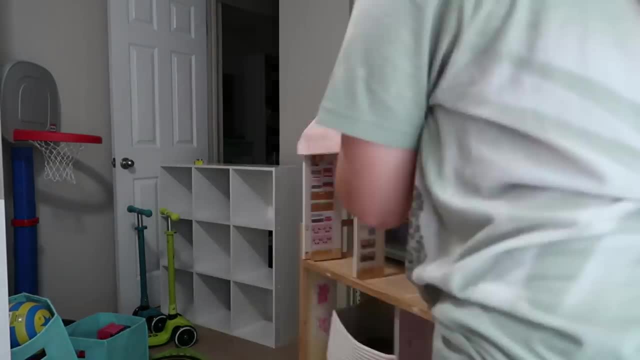 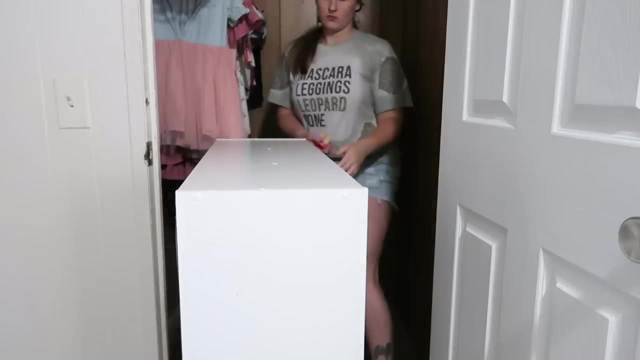 Now I'm moving over into their closet. I wish that I had a closet as big as a bedroom, because I could just shove everything in the closet, honestly. so I have to pick and choose what I'm going to be putting in the closet so that it isn't too much. so I did decide to put their 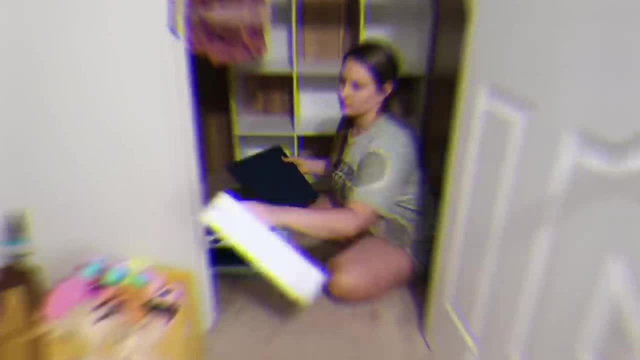 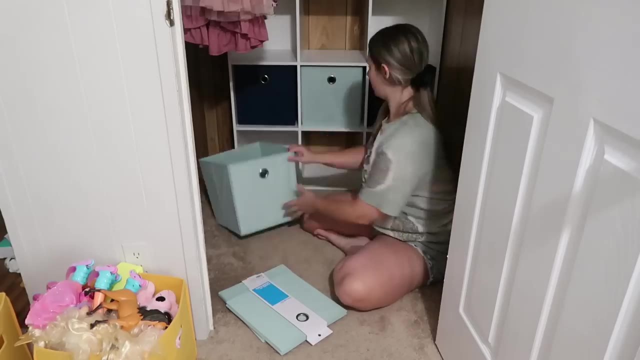 toy box in there and I am going to have to be replacing their cube organizers because a lot of them are ripped. They're just worn out and old from the last time I did their room makeover, just from having toys shoved in them. so I did pick up some new cube organizers. 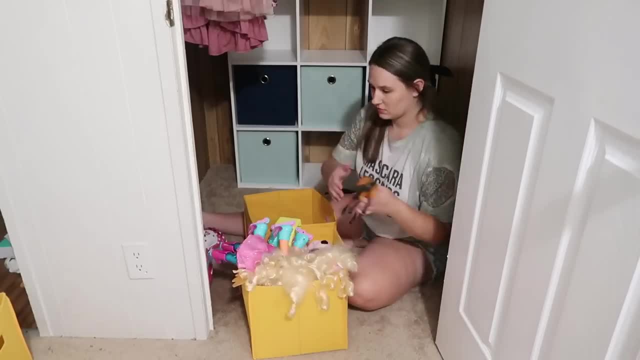 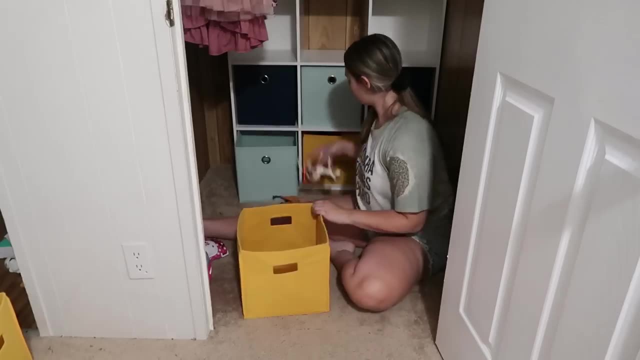 I wasn't sure if I wanted to still continue to use some of their cube organizers that were still in good condition, so I was trying to fit them in here and see how I liked them, but then I realized the design was different and it really bothered me. As you can see, some have metal circles. 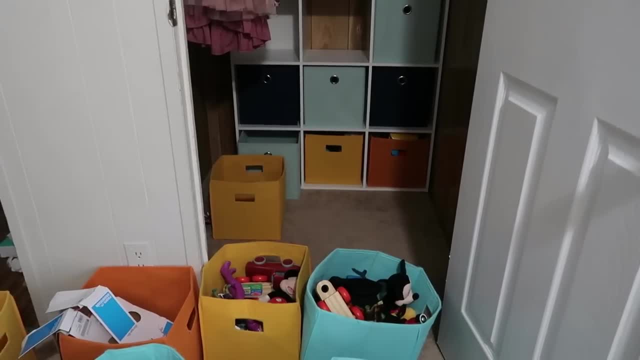 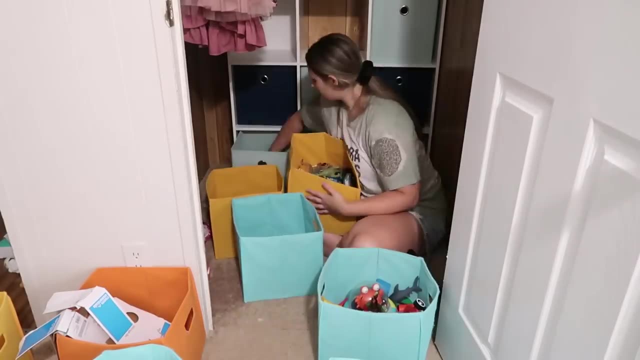 and then these just have like a cutout. so it just really bothered me, like an OCD thing or something. so I'm going to go ahead and go through all their toys. I am not decluttering their toys. I did not get rid of any of their toys. I just simply organized them in each container and the way I 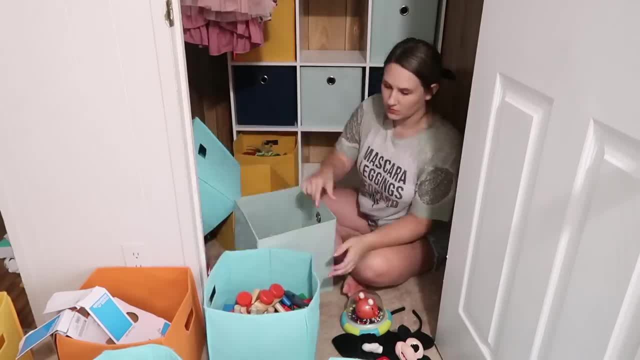 keep their toys to a minimum is by putting them in a box. I'm going to put them in a box and then I'm going to declutter through their toys about every six months, just anything that they're not really playing with. I'll either pass it down to Jackson and store it in his closet if it's too. 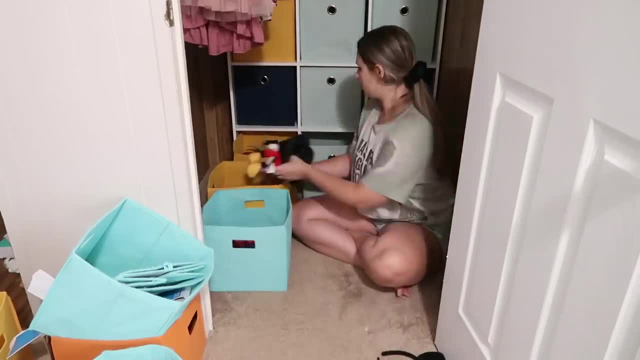 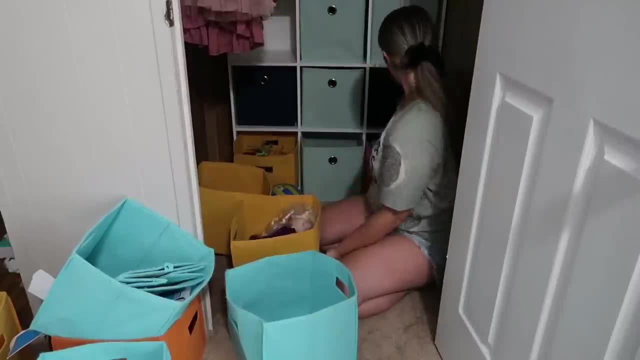 big for him, or go ahead and just put it in his room in his toy box, or I will just go ahead and get rid of it and y'all. toy rotation is a wonderful idea if you have a garage or someplace to store the toys, but unfortunately I do not, so that's why I don't do toy rotation, I just keep. 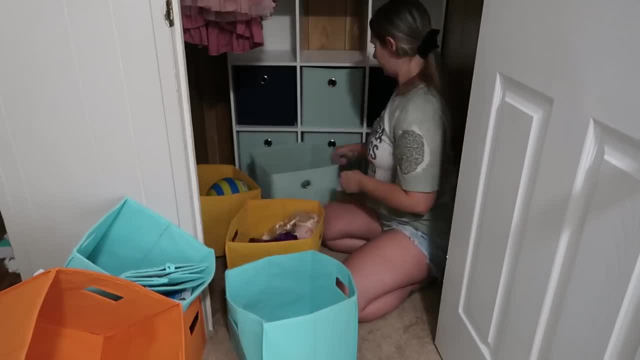 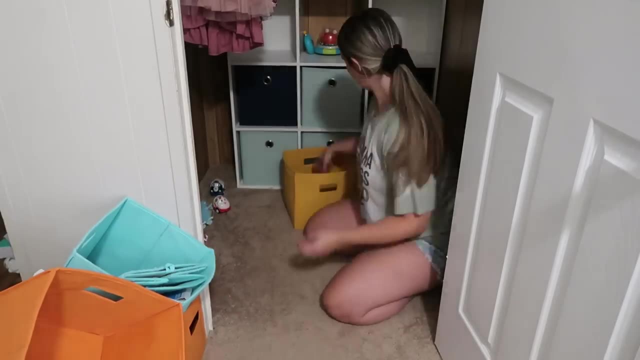 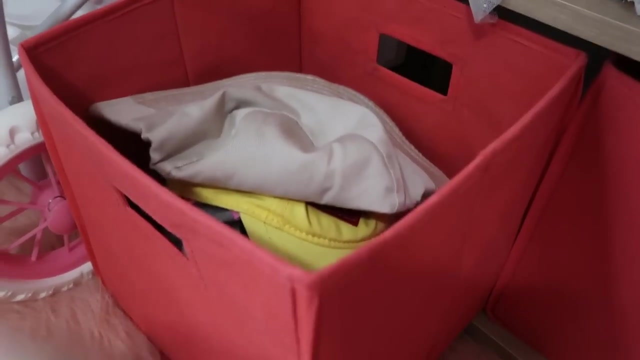 the toys at a minimal to what they actually play with. I found all of Nolan's Mickey Mouse ears and his hats and I'm going to be putting these in the dress-up display closet so that he can play with these with Arabella whenever they want to play. 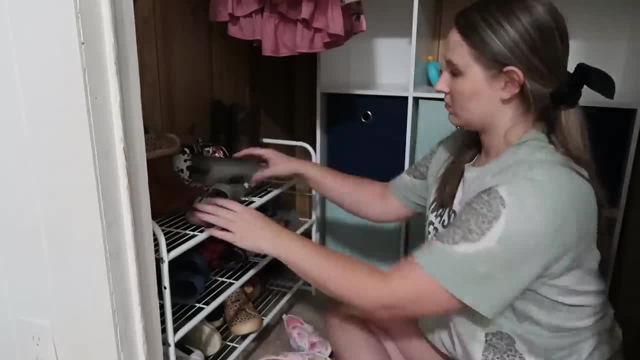 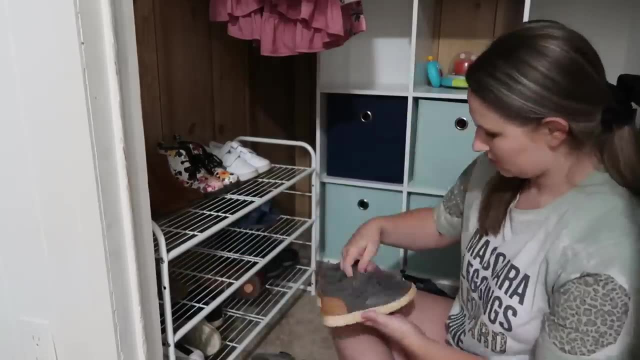 dress-up together and I'm also storing the Barbie styling head in the dress-up closet because she likes to dress it up with her bracelets and do its hair. so now I'm moving back over here into the closet. I'm just looking at all the sizes on the shoes and making sure they're all their sizes. 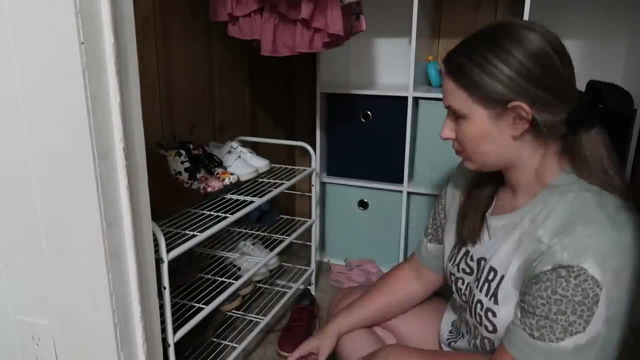 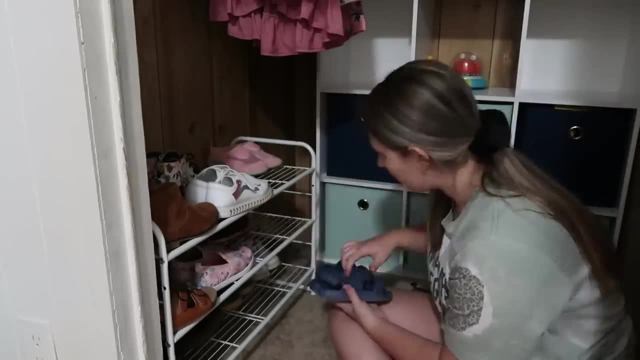 They have their play shoes and their nice shoes all mixed up here. They know what their play shoes are and they know what their nice shoes are. I always tell them their dirty shoes are their play shoes. but it's honestly very challenging fitting two kids' things in one bedroom, but somehow I 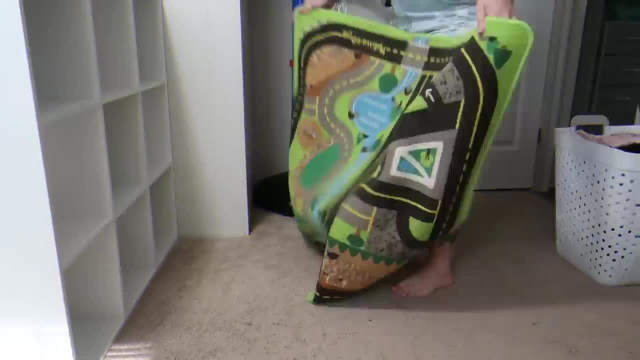 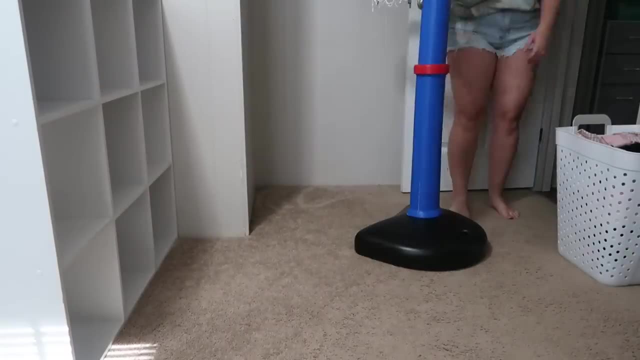 manage and I feel like I do a really good job at it. All the balls and baseball bat are going in the rope basket in the closet. I'm going to be shaking off the Melissa and Doug play mat. It is just a road map that he got for Christmas and he absolutely loves it, so I'm going to be making a. 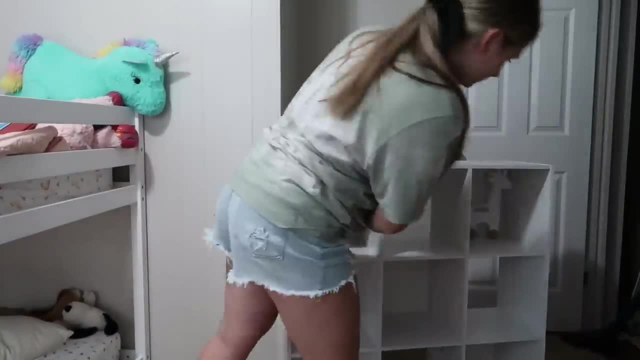 space for that kind of like doing centers in their room. this time, Instead of doing corners, we're going to be doing centers. As for the top of the display: closet. I thought it'd be cute to put all their stuff in there, so I'm going to be doing that. I'm going to be doing the display closet. 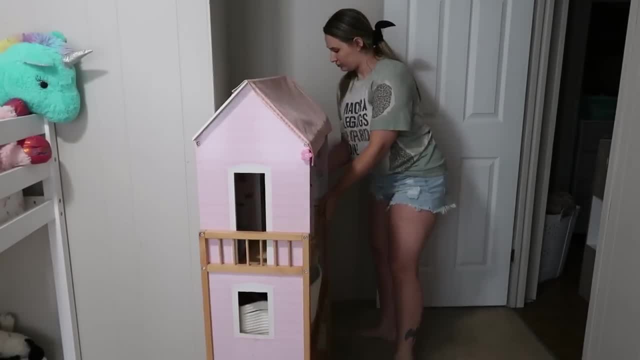 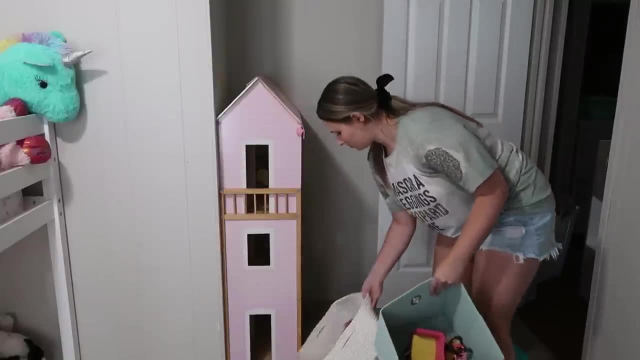 small stuffed animals up here and Arabella's wooden little rainbow. and I found the most perfect place for Arabella's dollhouse: right here. When you first walk in. it fits perfectly right here in this space. and for all the Barbie furniture and Barbies. I keep them in a container. 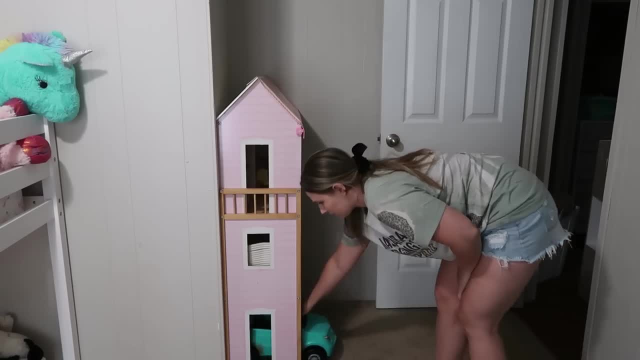 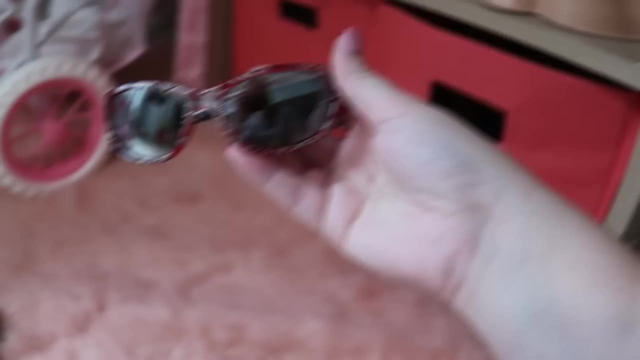 inside the dollhouse so that she can just take them out and play with them when she wants to play with them, and that keeps them really tidied up. It's very challenging fitting all the large size toys in here when we don't have a playroom, but I'm so thankful that we have the space to fit. 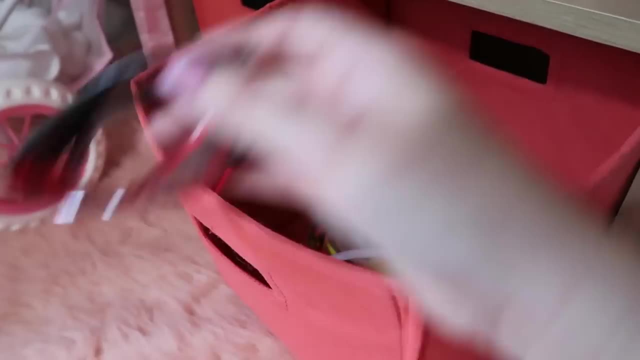 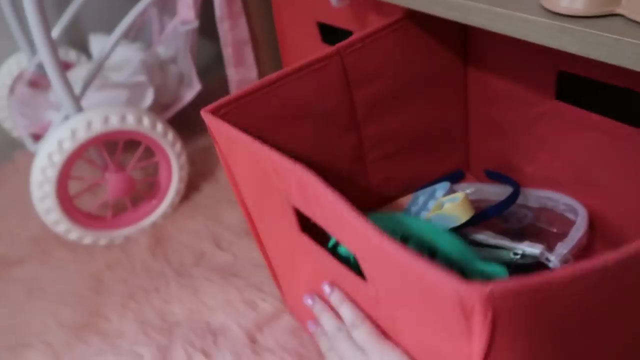 everything. These are Nolan's absolute favorite sunglasses. He loves his Spider-Man sunglasses. So the two bottom containers are going to be headbands, hats, sunglasses. these little poppets, just little tiny things are going to go in these cube organizers and I think it's a really good. 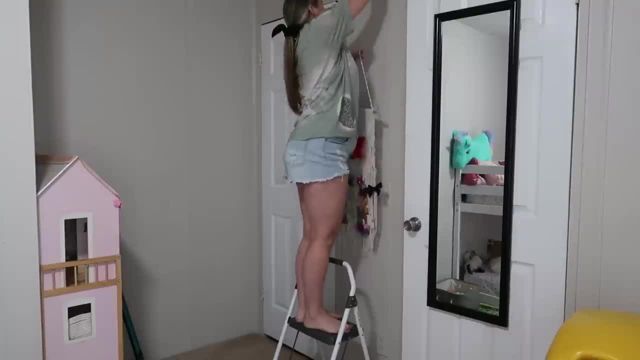 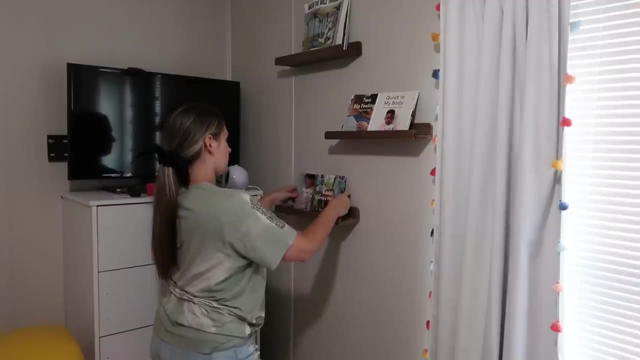 way to organize them. I decided to move Arabella's bow holder over here in this space and I think it looks so perfectly over here and it's easier to grab a bow instead of walking in and going across the whole room, I can just walk in and grab one right there by the door. I also have 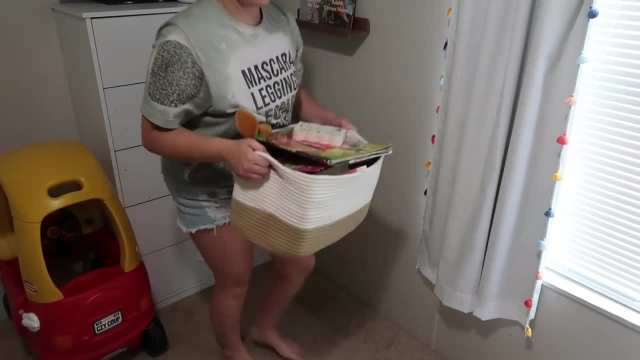 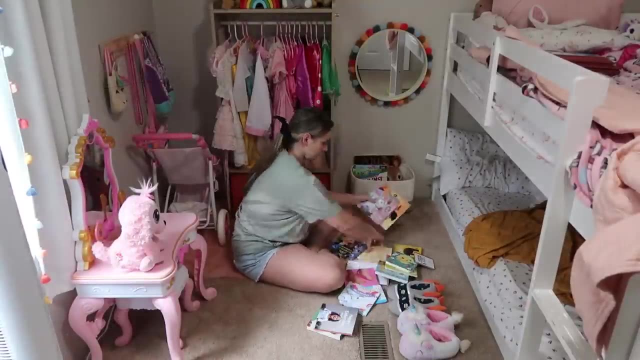 this book display in here. I just switch out their books every week so that they can have different books to look at, but I just think they're really cute up on the wall. I'm going to go ahead and and I have them high because I felt like they would try to climb up them, so I just have them. 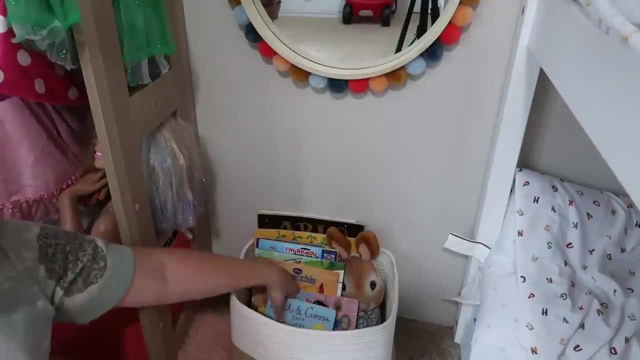 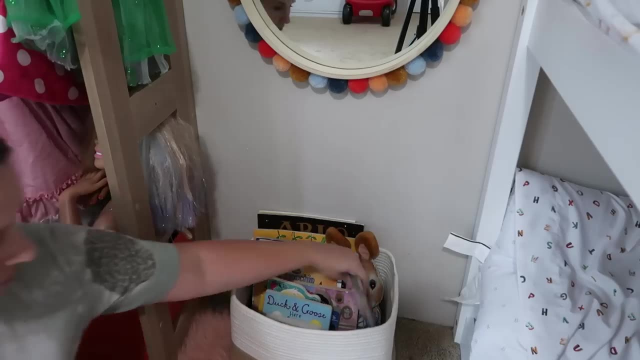 up high and it just makes a really cute book display. Over here underneath their mirror. I have a basket where I'm going to be putting all their other books, and I actually ended up having to get rid of a lot of books that were just damaged, ruined, ripped, so I'll be going back. 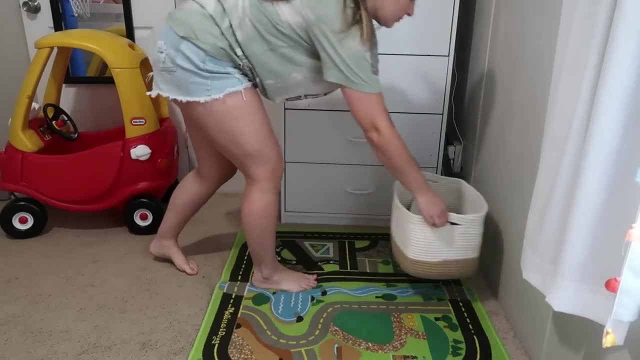 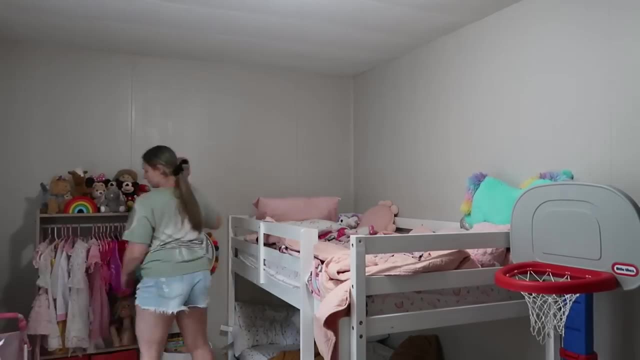 to Rawls and getting them some more books. I love getting their books at Rawls. They're so affordable there. Over here in front of the dresser, is going to be the car center I mentioned earlier. I was doing centers, so towards the end of the video I'm going to do a little bit of a tour and I will 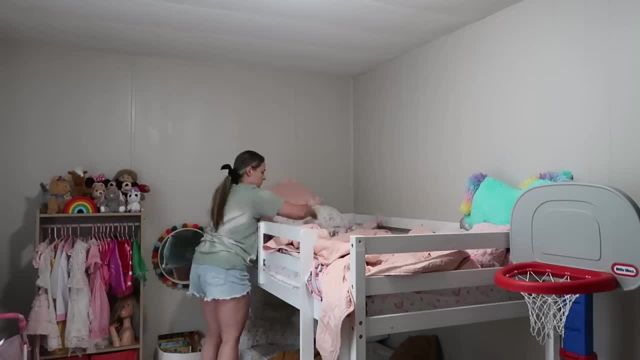 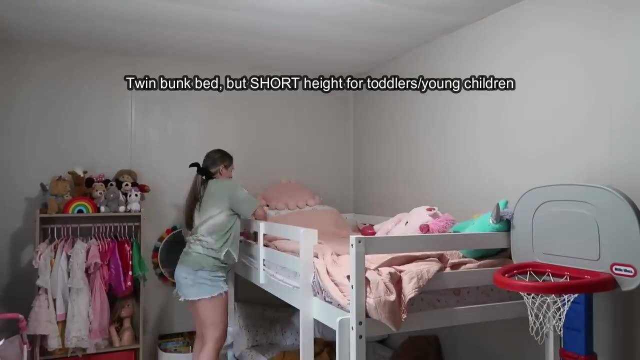 the centers later on. And lastly, I'm going to be making up their bed. I don't usually make their beds all perfectly, because it is very challenging with this small toddler-sized bed. The bottom is so small to crawl into and it's really hard to make this bed up, honestly, so I kind of just slap. 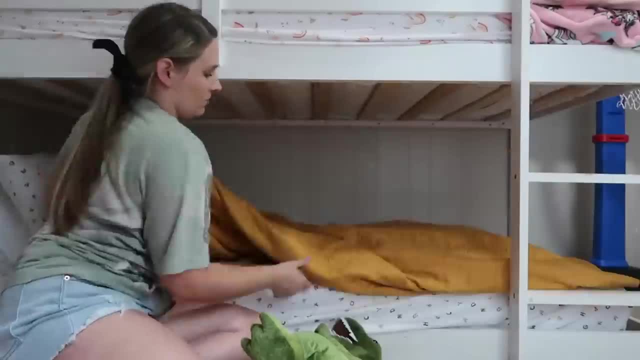 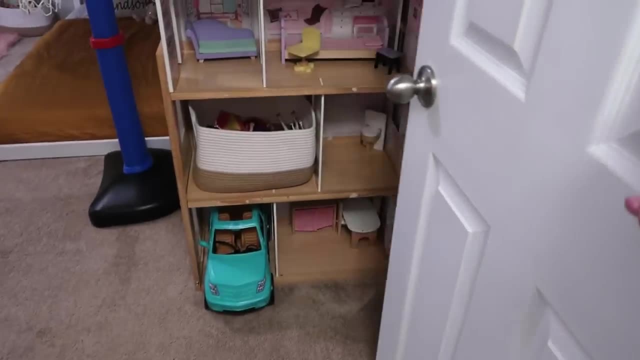 their blankets on there. They get in there and lay in their beds and mess their blankets up during the day anyway, so I'm not too worried about it. I'm also taking down this closet mirror, since I did get them the pom-pom mirror, and now I'm going to go ahead and show you guys all the afters and 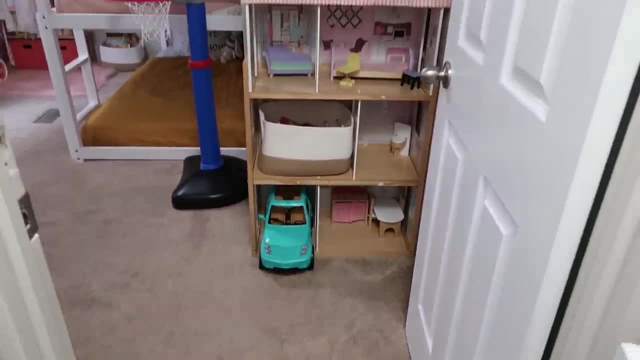 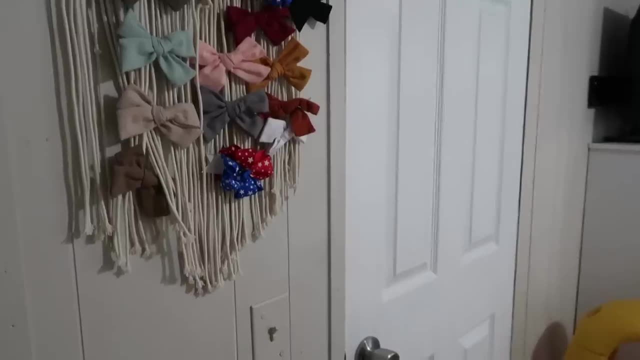 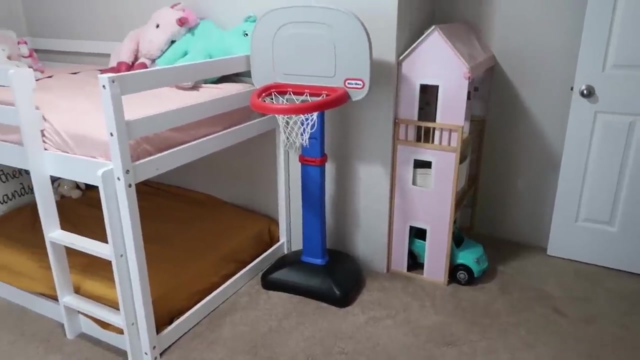 do a bit of a tour. I'm going to go ahead and show you guys all the afters and do a bit of a tour. The best place for the dollhouse and the basketball goal was right when you first walk in and there's. 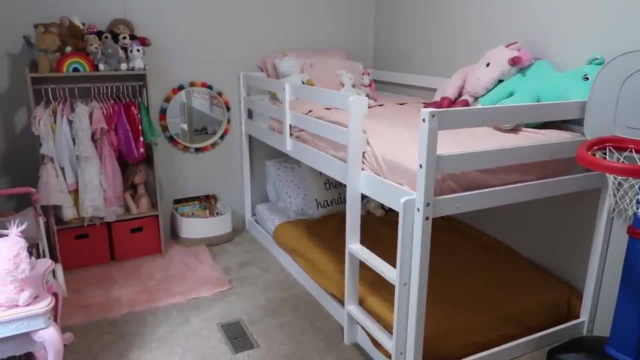 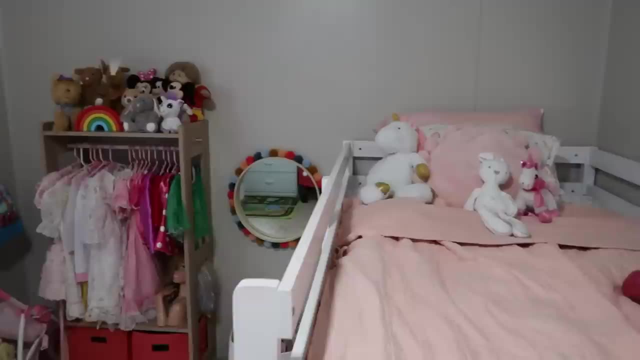 plenty of space for them to play with both of those toys. So right next to their bed is their dress-up center, as well as their reading center. This is where I have their books and they can play dress-up together, and I can't wait to get some more dress-up costumes for little boys to go in here. 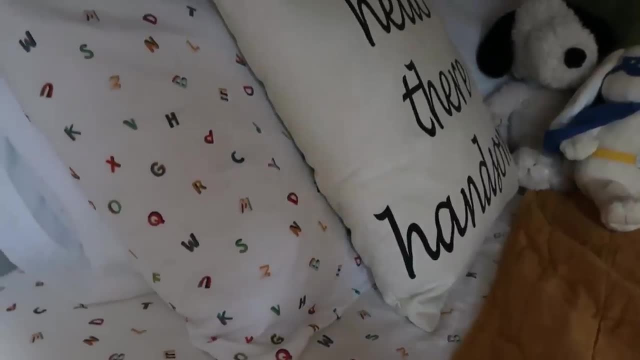 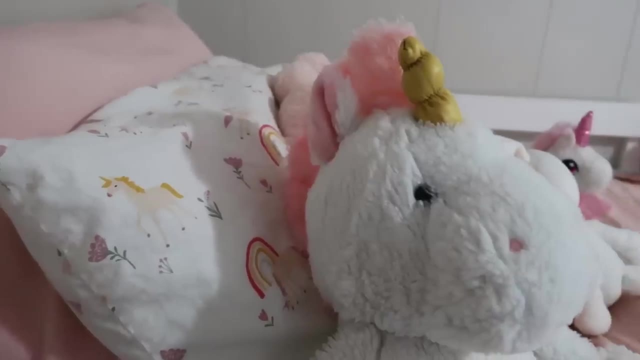 Now that we have the space for it. it's going to be so much fun. I've had this Hello There Handsome pillow in Nolan's nursery when he was a baby, so it's super sentimental. and then I just love Arabella's unicorn and pink up here on her bed. I love that the pom-pom mirror is down low for. 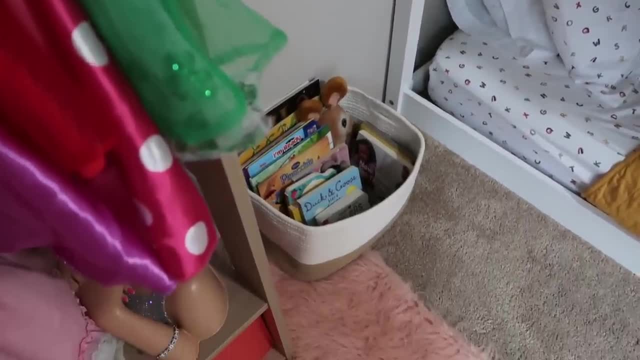 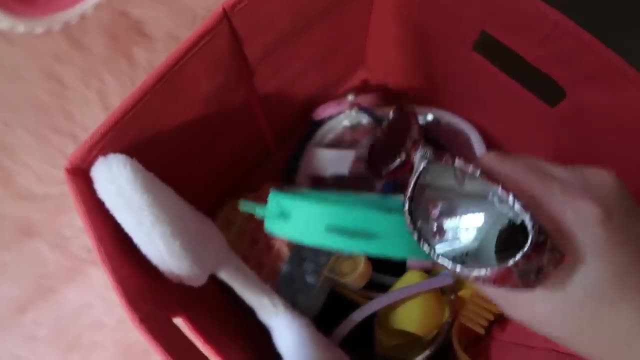 toddler height. for small child height It is so adorable so that they can play dress-up and look at their self in the mirror. The two storage bins under the dress-up display are not going to be in order. These are just to hold all of their sunglasses and their pop-it toys. It's got. 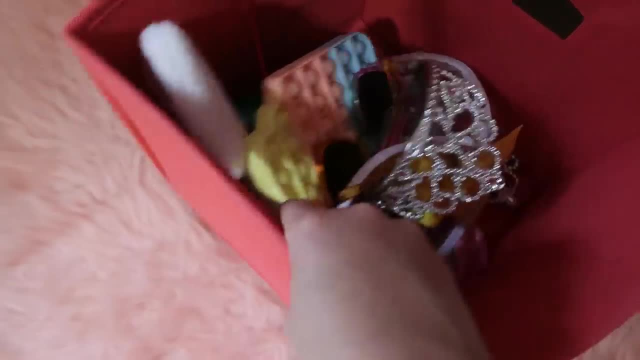 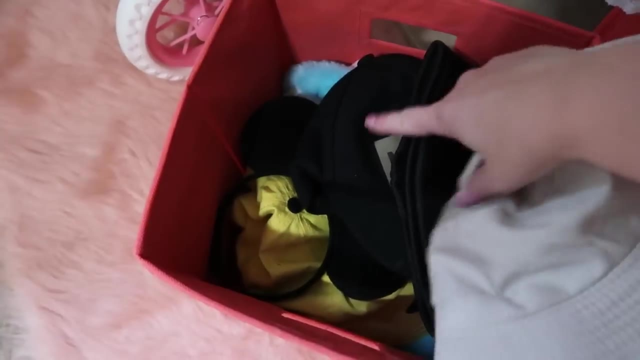 Arabella's crowns and headbands. There's some Easter bunny ears in here, just fun dress-up things. The other one has a lot of Nolan's Mickey Mouse ears and his hats in this one and some of Arabella's hats, so I really love that I was able to combine all of these and just make it really. 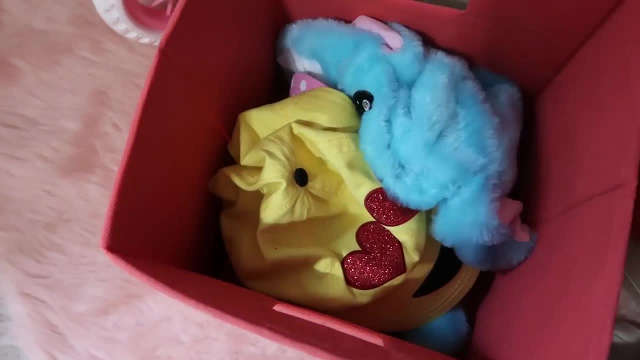 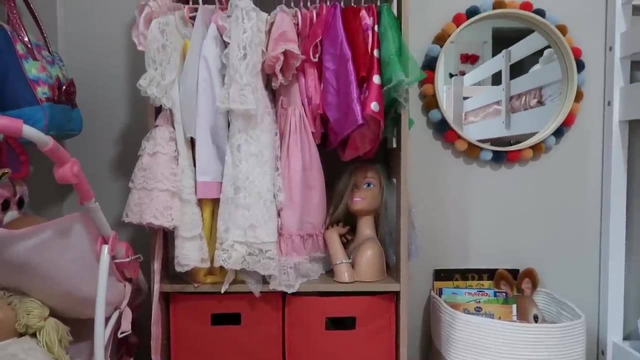 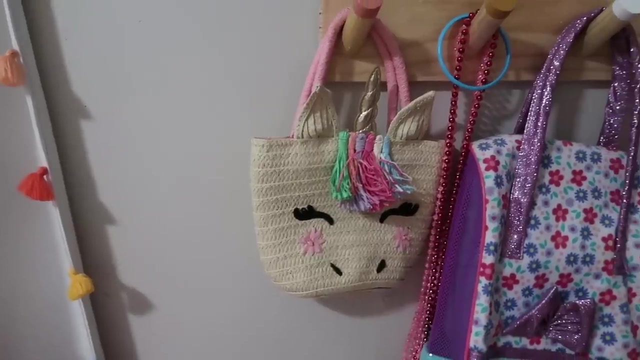 fun for both of them And they are more than welcome to grab their stuffed animals and play. That's just where I stored them. This little rack here is from Target from the last time I did their room makeover and it's just going to be holding all of the purses, necklaces and they can also. 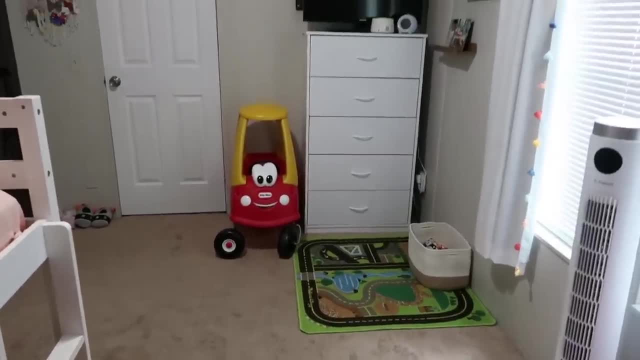 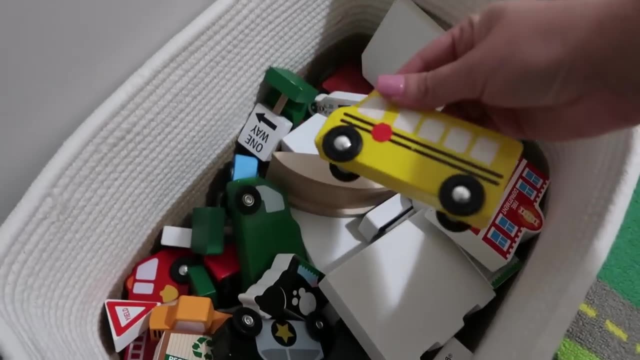 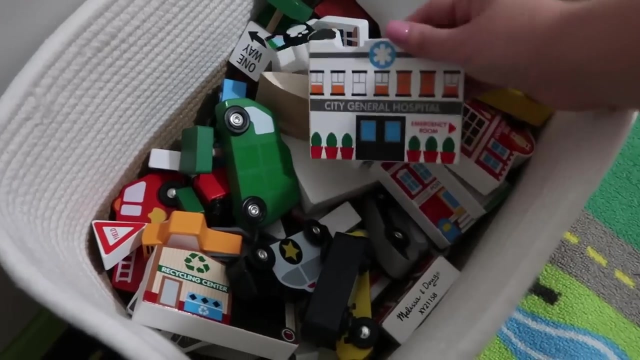 hang their hats on it. Over here in this center is going to be their car center, their city center. So this container has a lot of little wooden cars and wooden pieces that go to the road map. There's a hospital and a recycling center, police cars, fire trucks- all the things that you would 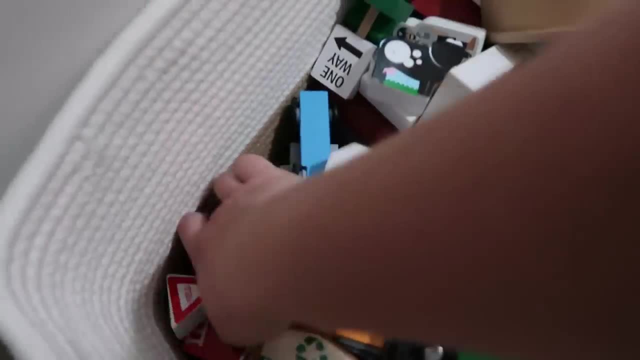 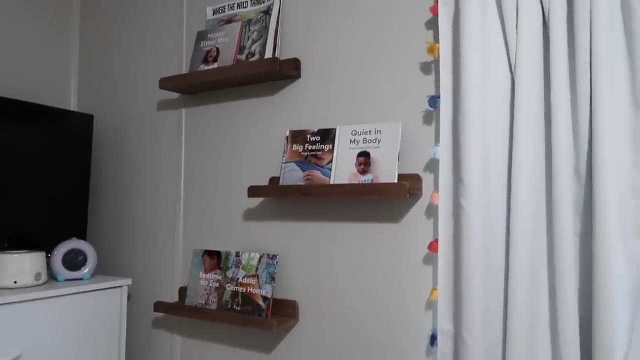 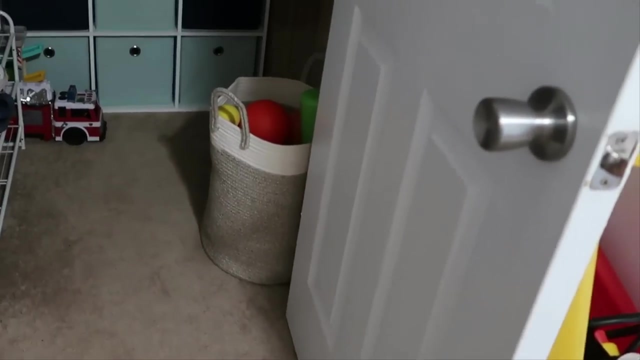 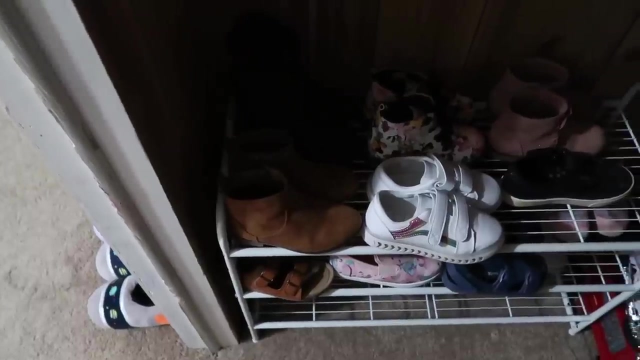 need. There's a little bridge, a school, little yield signs and stop signs and little police officers. It is so cute and they just love to play with us together. So I decided to downsize from two cube organizers to one cube organizer in here and it has made a ton of extra space. 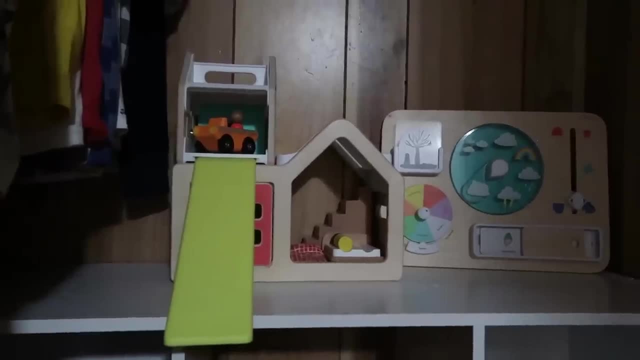 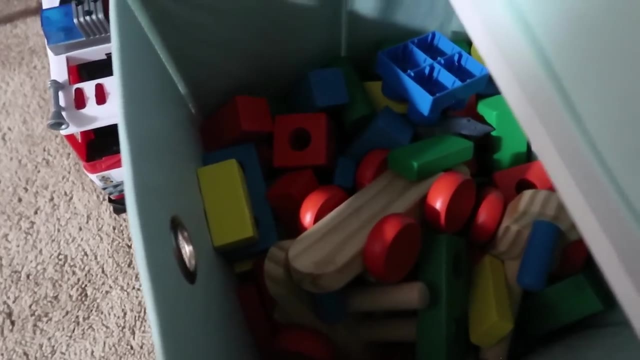 And all their toys fit perfectly with extra storage In this cube organizer, with just having one. so it is perfect. I do have both of their toys in this cube organizer, but they are organized. So these are the wooden blocks. I also have one of just. 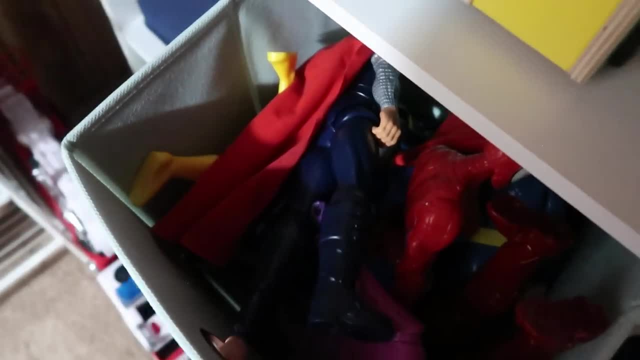 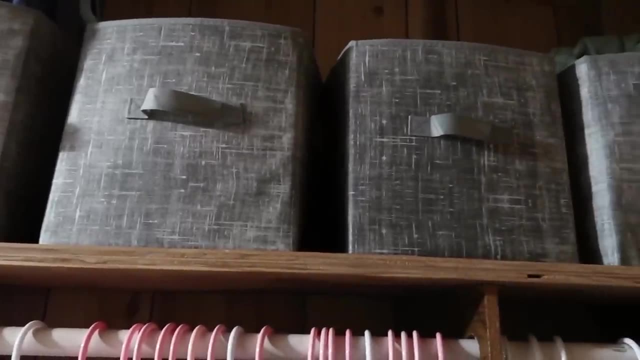 Arabella's princesses and her ponies. This one is full of action figures and superheroes. This is all the mega blocks, so on and so forth. On the top of their closet I have all of their winter clothes that they are going to be fitting into this year, as well as Arabella's book bag and 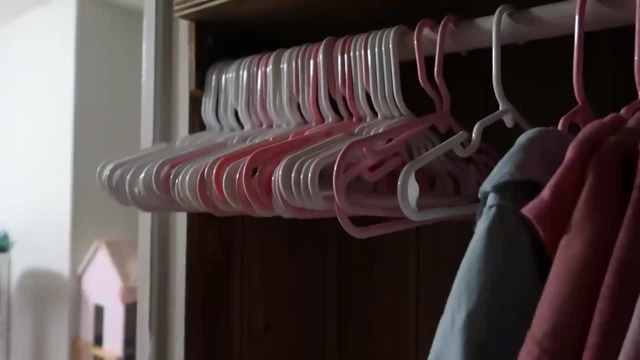 her nap mat for pre-K. this year I have all of their clothes that they are going to be fitting into this year. I have Nolan's clothes in the back of the closet. Arabella's are in the front. I also have some pink and white hangers for them. Nolan uses the white ones and Arabella uses the pink. 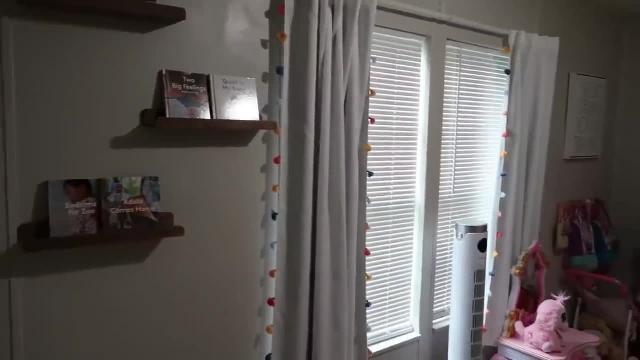 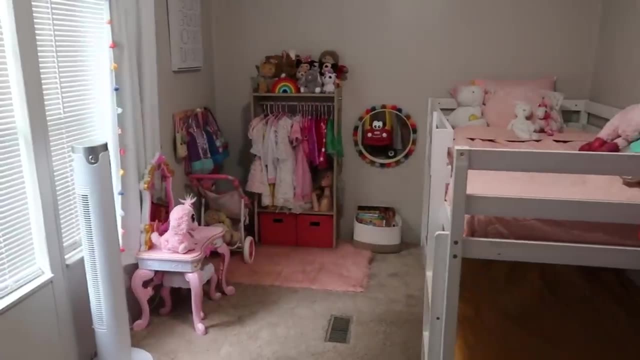 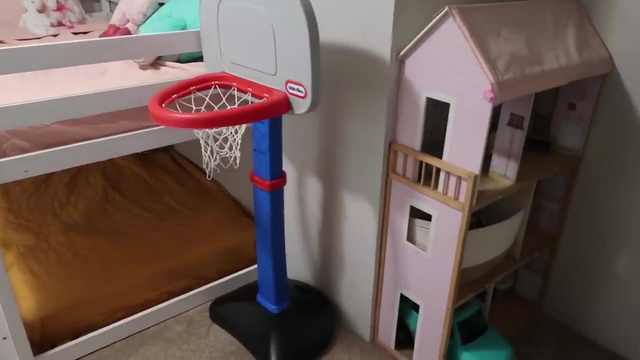 ones. My ultimate goal is to make this room fun, bright and colorful for young children. I don't want it to be super neutral just because it is a shared room. That is why there are so many colors in here, and I absolutely love the way that it turned out. So now let's go ahead and surprise. 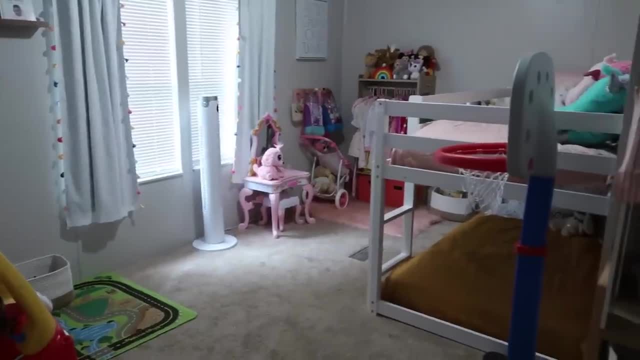 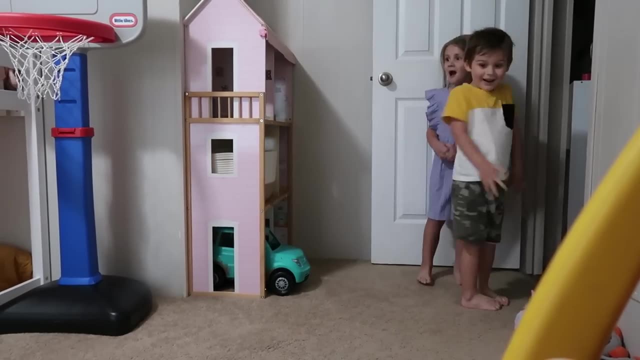 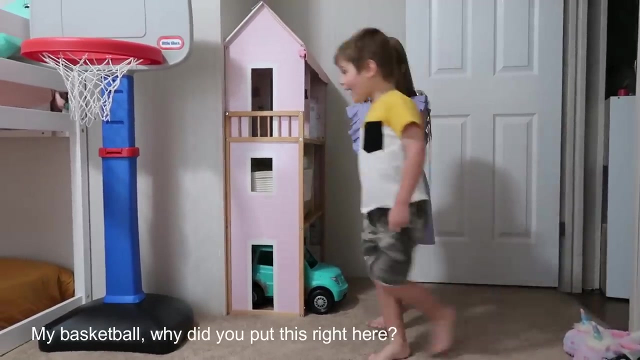 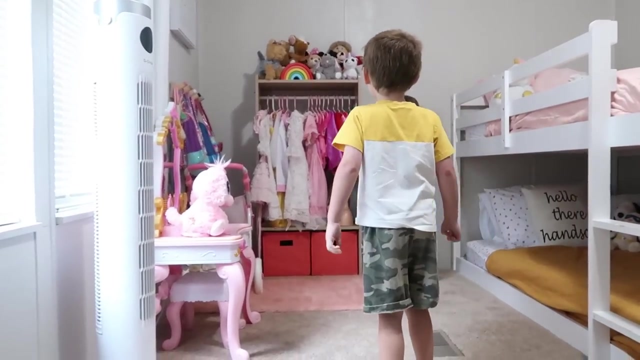 their new, freshly cleaned organized room and show them their new dress-up display shelf and get their reaction. Okay, you can look. Look over there, Nolan, All your Mickey Mouse hats are over there and the stuffed animals and the books. That's for Bella and for Nolan. 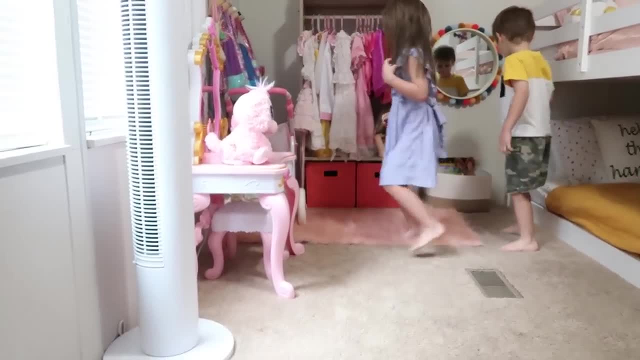 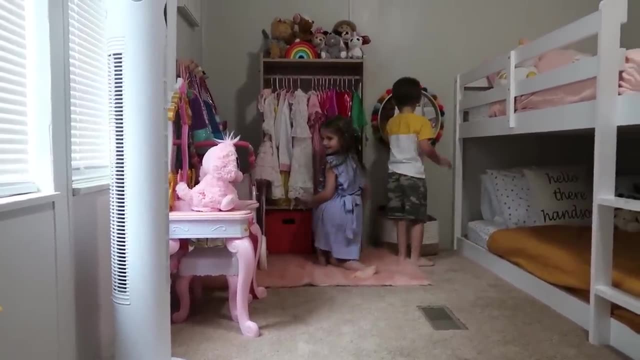 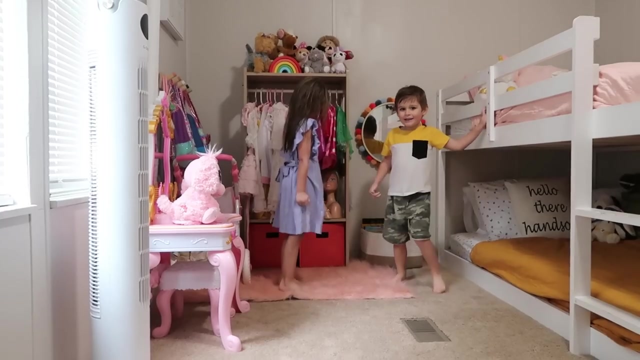 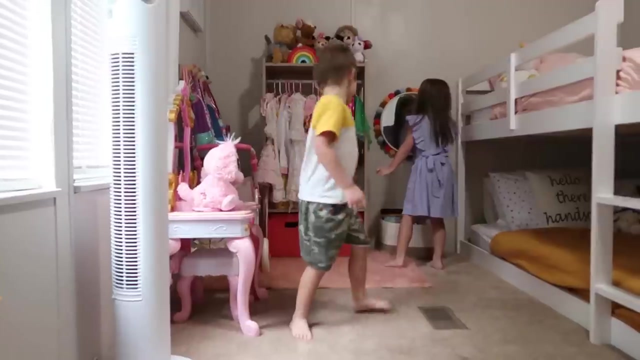 Look down there. Look down there in the boxes. Your Mickey Mouse ears are in the boxes. It's got pom-poms on it. You love your room. Did you find your Mickey Mouse ears? It's in the pink boxes, The pink boxes. 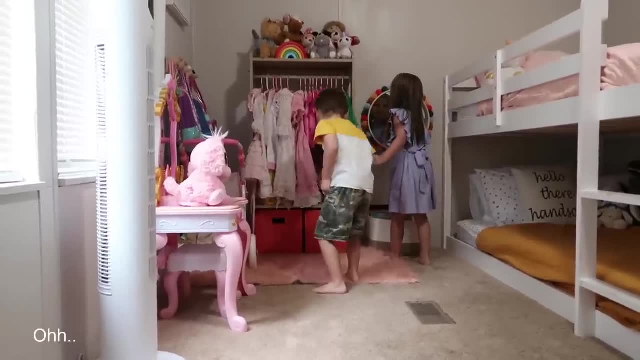 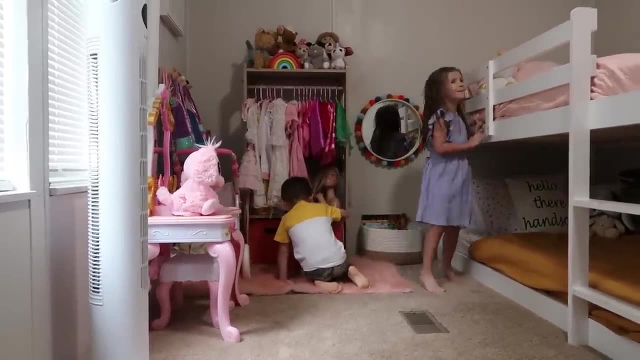 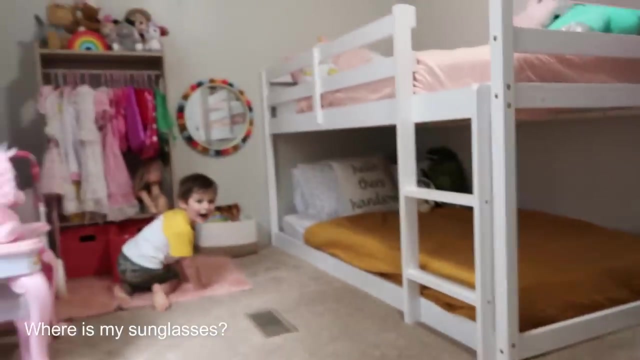 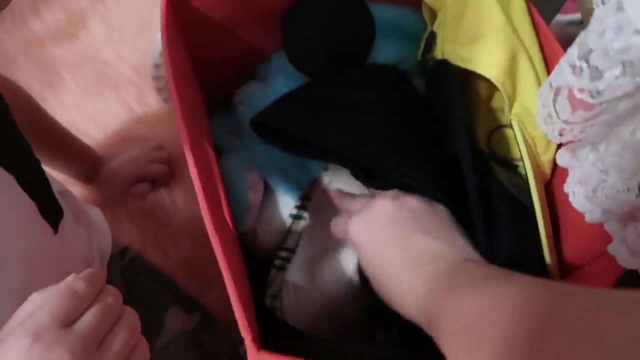 Where is it You got your sunglasses? You got your sunglasses in there and all your Mickey Mouse ears. Wow, Wow, Aww, I love you, I love you. What's in there? You've got Nolan's hat and your Mickey Mouse ears- your other hat. 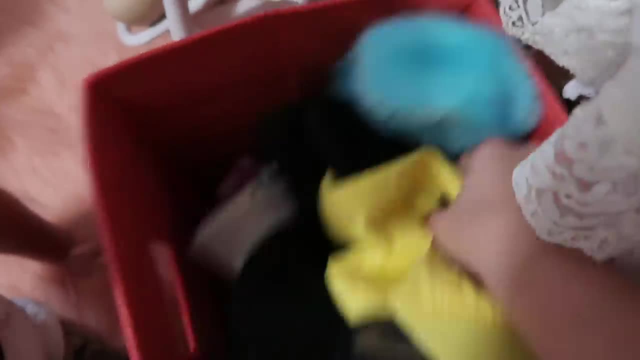 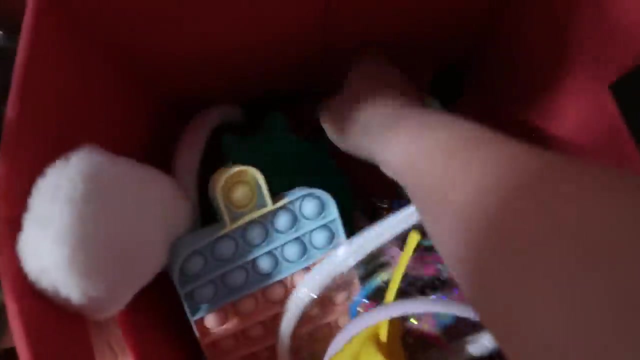 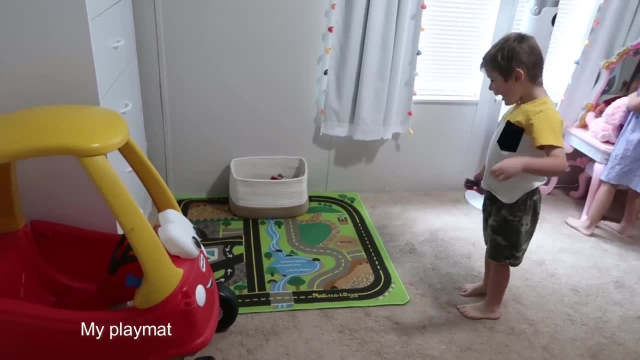 Nolan, what's over here? My play map, Your play map. What's in there? Is that all the pieces, so you can find them all easy? Y'all didn't even see the closet- yet A closet. Let's look at the closet. 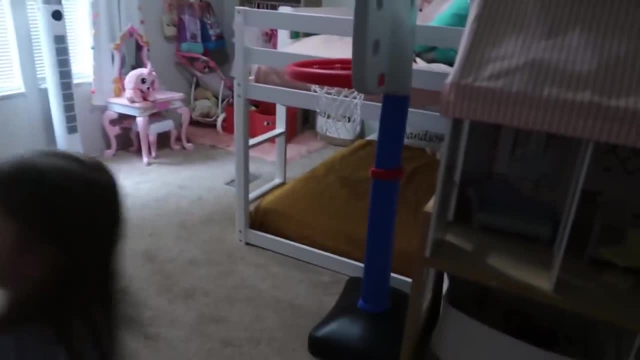 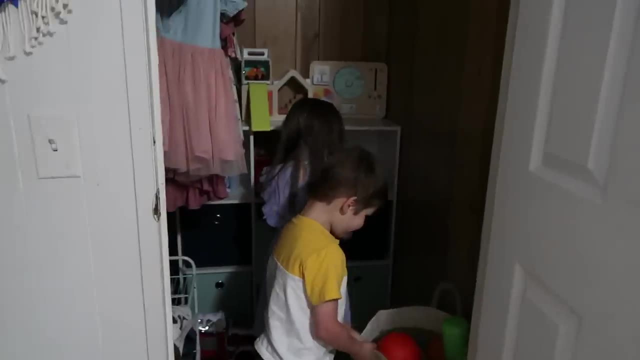 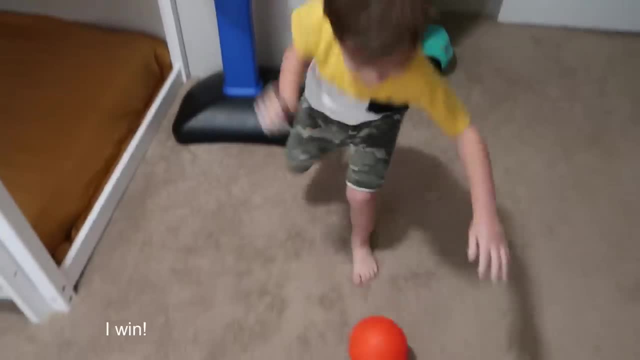 That's mine. That's mine. Take that up. That's mine. My toy box, Oh and my. I like them. That's your toy box. That's gonna be where we clean up all the toys. Jackson's waking up from his nap. 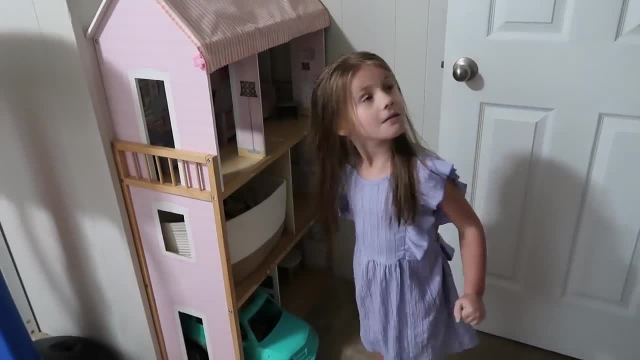 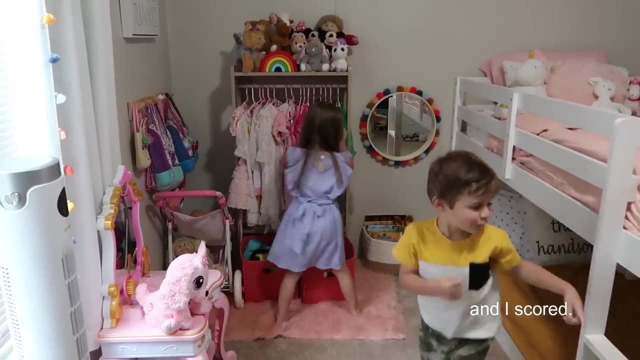